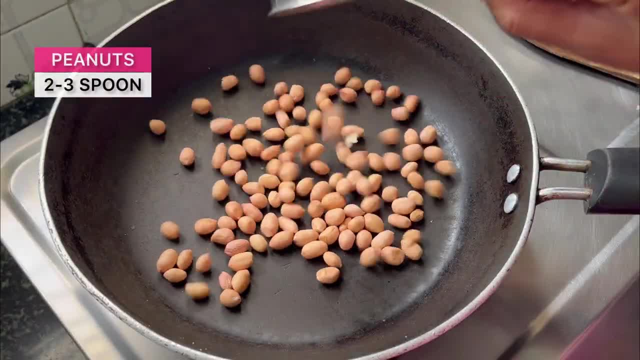 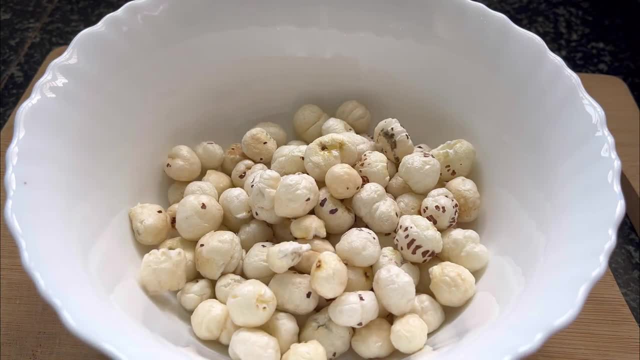 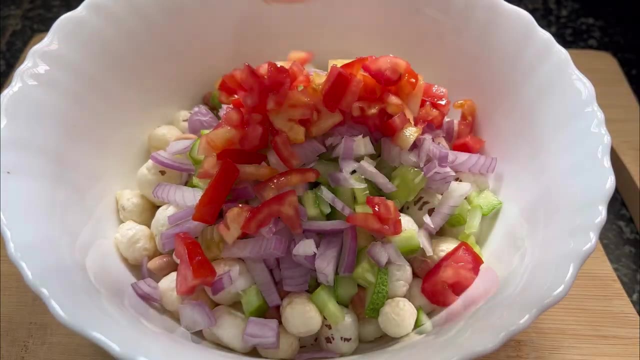 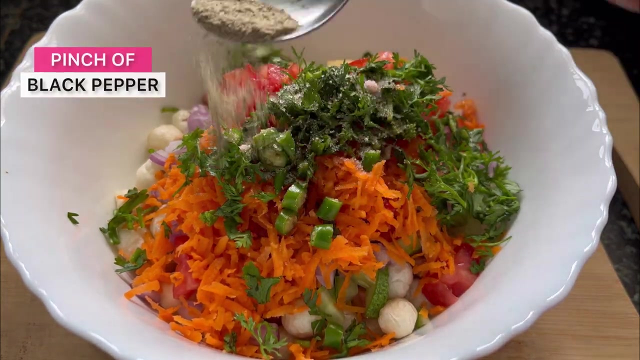 it gets crunchy, Add some peanuts and roast it as well on low flame. Now in a mixing bowl, add roasted Makhana roasted peanuts. add chopped cucumber, onion, chopped tomato, grated carrot, coriander leaves, chopped green chilli. add rock salt, pinch of black. 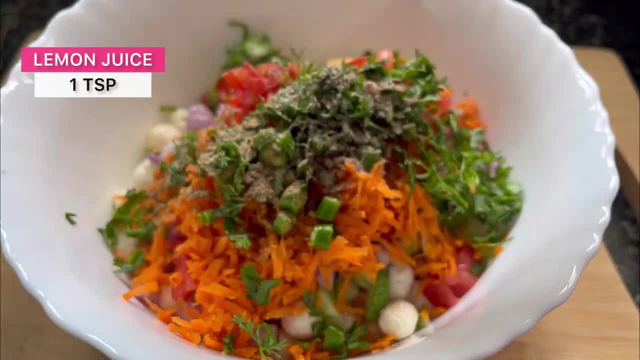 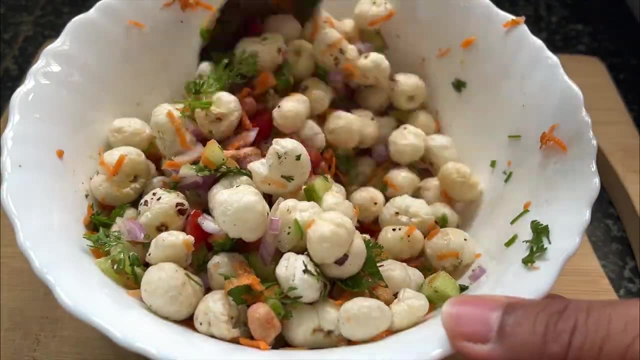 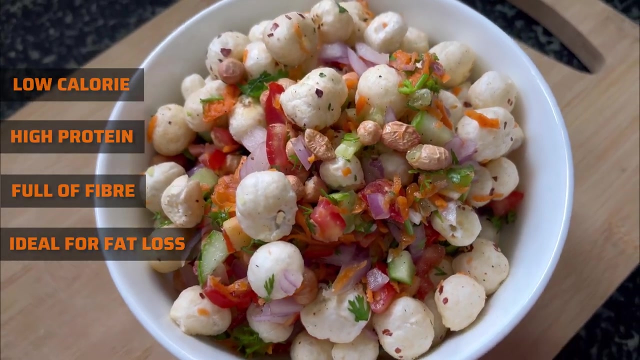 pepper, half teaspoon chaat masala and 1 teaspoon lemon juice. Mix it properly and your super crunchy Makhana Chaat is ready to be served. Super low in calories, yet full of protein, fiber, iron and other micronutrients, This snack is best. 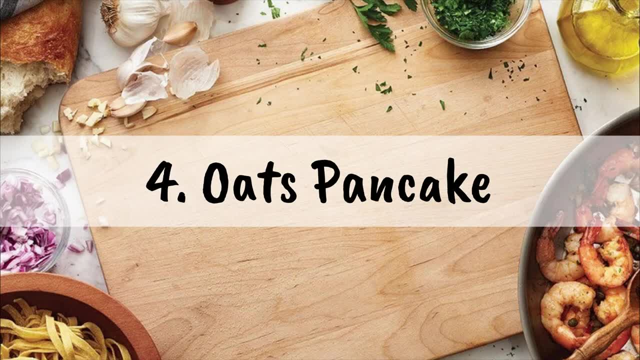 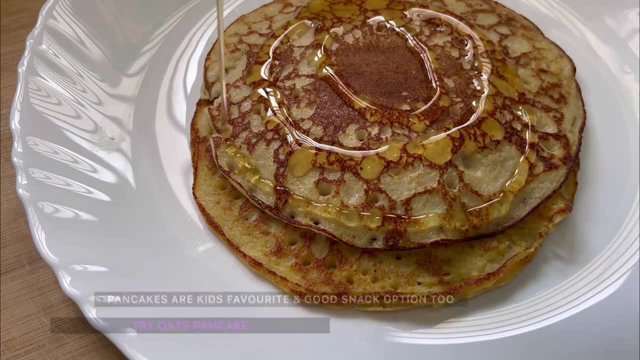 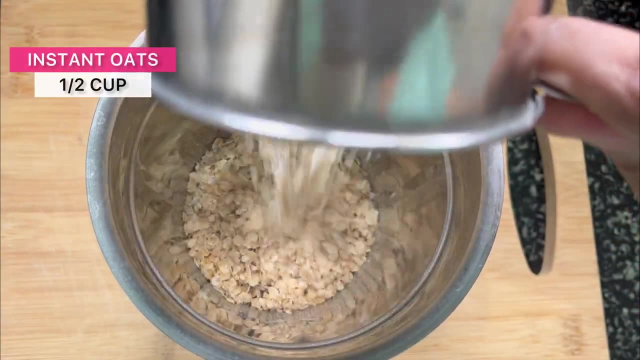 for weight loss. Number 4 on the list is Oats Pancake. This high fiber pancake is quick to make, healthy and amazingly tasty. My son loves them to eat. This is a good tiffin box option. also, To make it in a blender, take half cup instant. 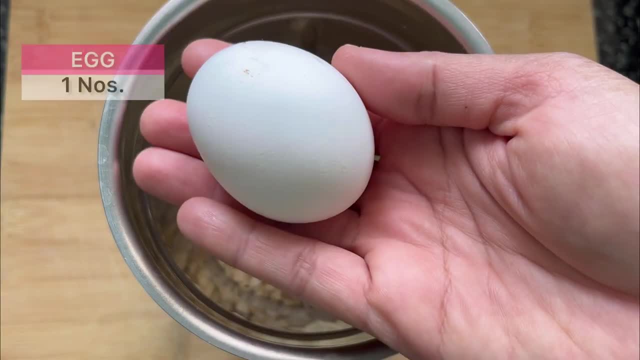 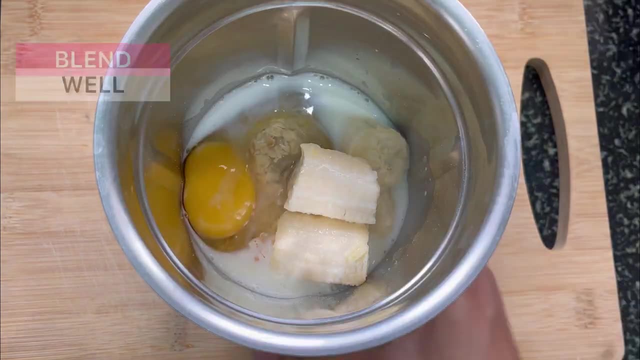 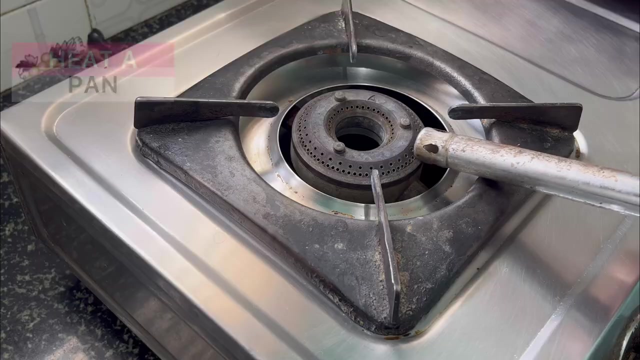 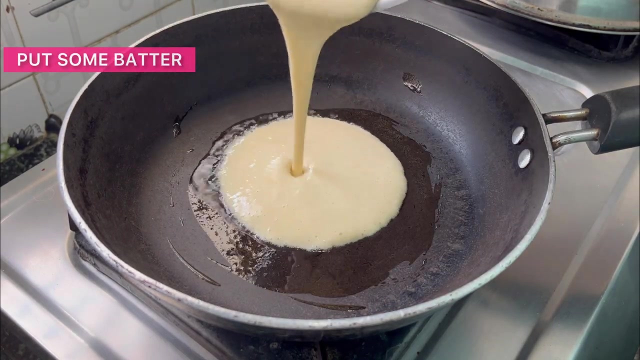 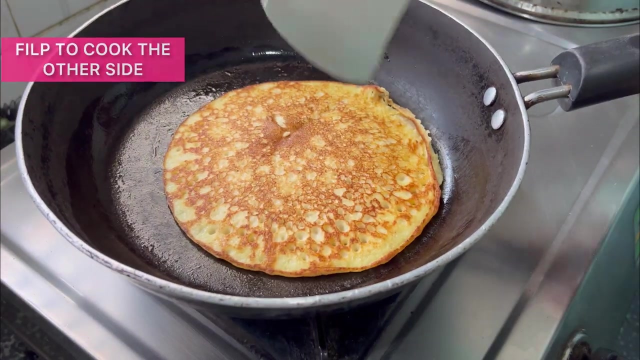 oats, add one or two ripe banana, one egg and half cup milk. That's it. Blend it well. This is the perfect consistency. Now heat a pan, put some ghee on it. Now add some batter and close the lid. Cook on low flame for 30 seconds. Now flip it to cook the other side. 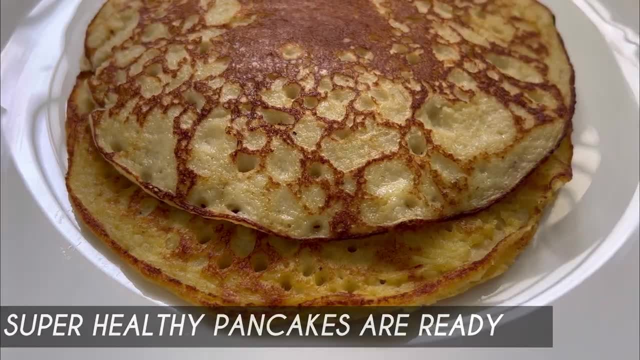 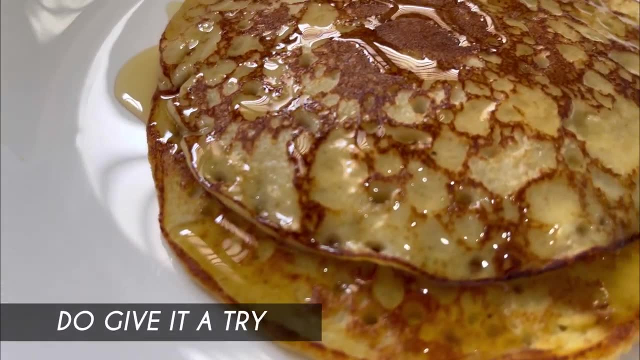 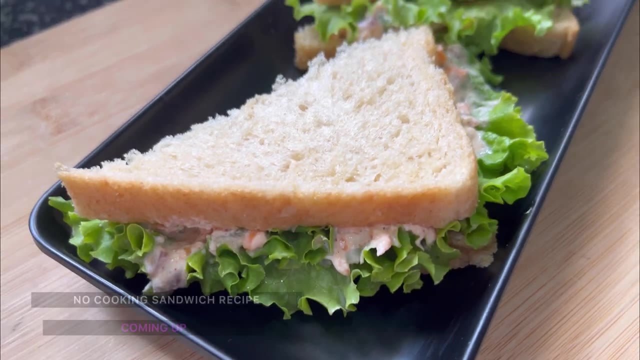 That's all. Your healthy oats pancake is ready. Finally, drizzle some honey on it to enhance its taste. Number 3 is Curd Sandwich. A snack option list is incomplete without a sandwich, isn't it? And if you do not have to cook it, then nothing like this: You'll get a perfect sandwich. 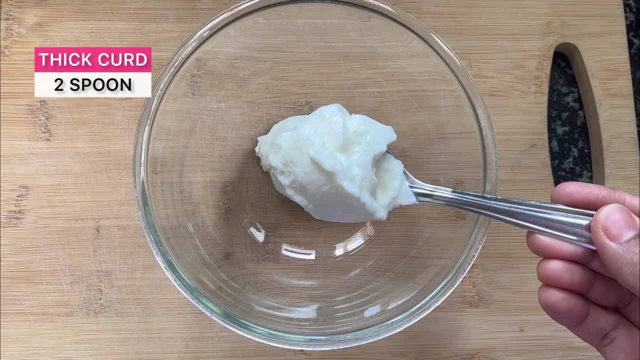 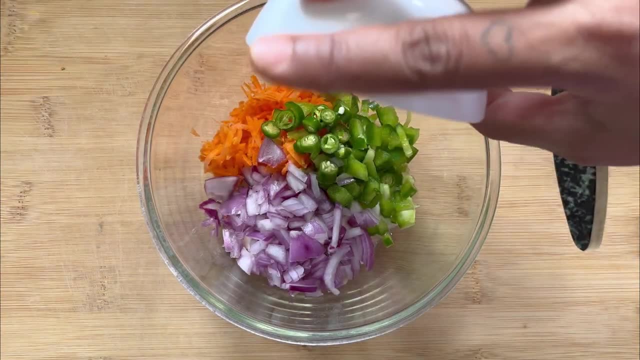 You can make this, You'll get a perfect sandwich. And if you have to go for a quick fast and like it in a mixing bowl, take 2 spoon of thick curd or yogurt. add grated carrot, chopped capsicum, onion chopped, green chili. add salt to taste. pinch of black. 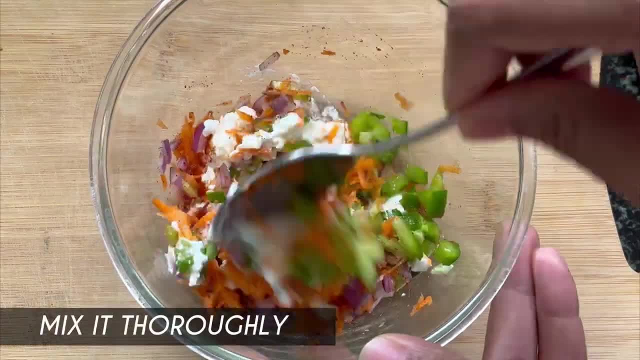 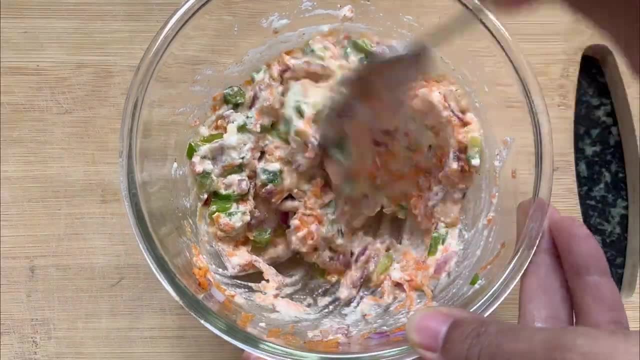 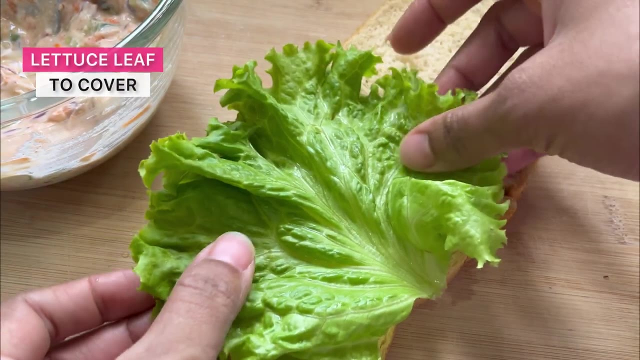 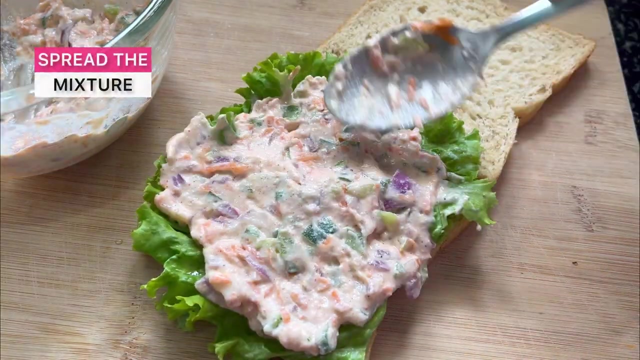 pepper and half a teaspoon chili powder. mix it thoroughly. now add cheese. this is totally optional. mix it well. now take 2 slices of whole wheat or atta bread. take lettuce leaf and place it first on the bread so that it does not make your sandwich soggy. now spread the mixture on it evenly and sandwich it with other. 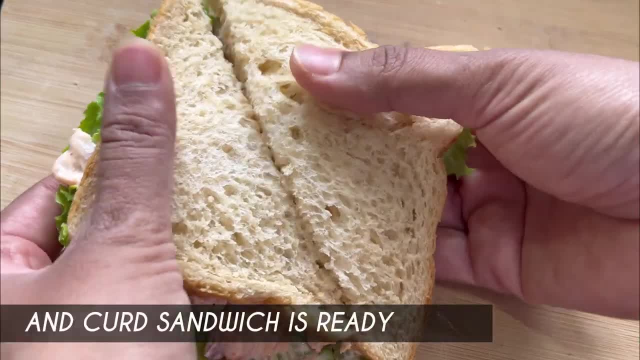 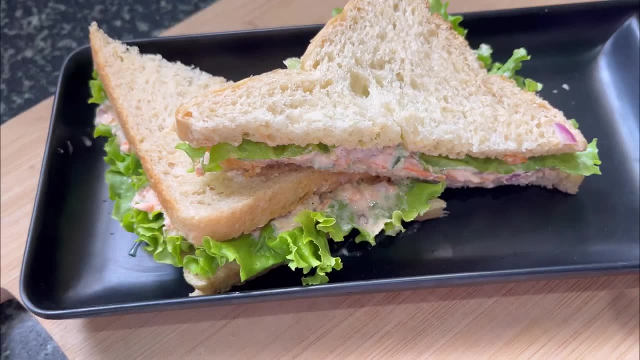 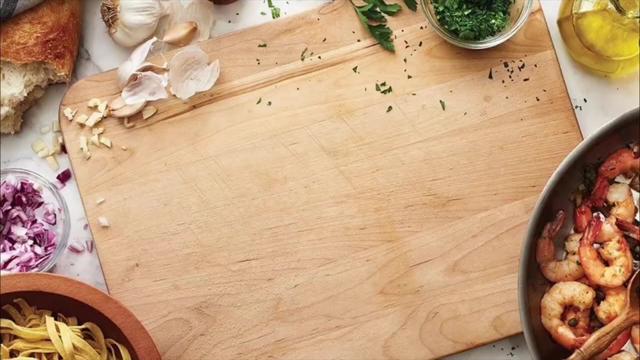 slice of the bread and cut it them half and your curd sandwich is ready to be served. this healthy sandwich with the goodness of raw veggies is highly nutritious and the taste is just awesome. give it a try. just make sure that you choose whole wheat bread. number two is 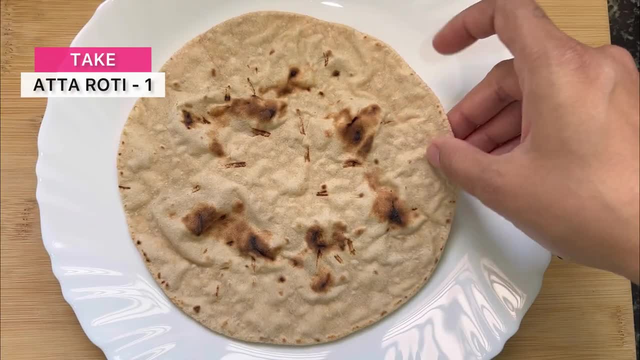 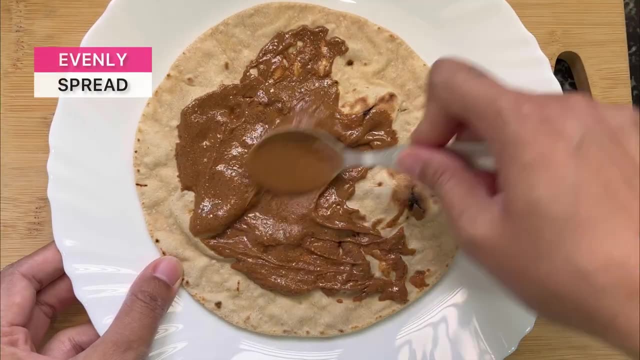 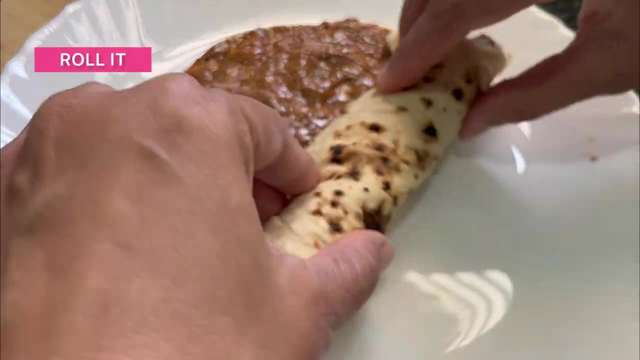 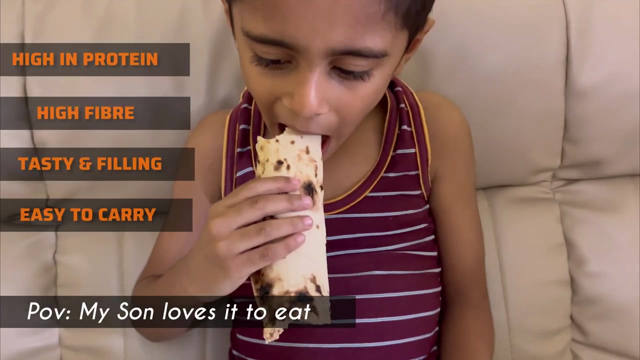 the bread of your choice: banana, peanut butter roti. simply take one whole wheat roti or atta roti. on this, take one or two spoon peanut butter and evenly spread on the roti. top it up with the slices of banana, roll it. that's it. your banana peanut butter roti is ready. well balanced with complex carbohydrates. 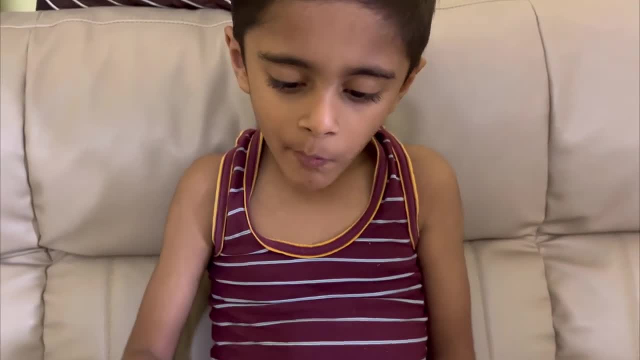 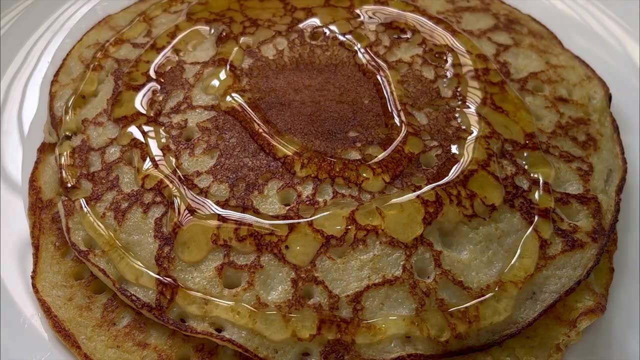 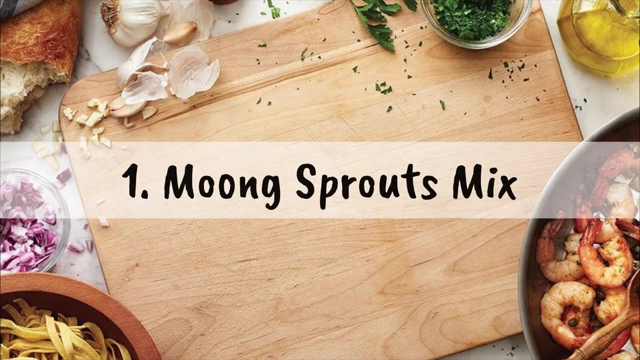 proteins and healthy fats. this snack is surely a treat for the sweet lovers. now, before i reveal my top pick, number one recipe, i want to quickly mention that fresh fruits are always good option for snacking. coming back to number one option, which is moong sprouts mix. 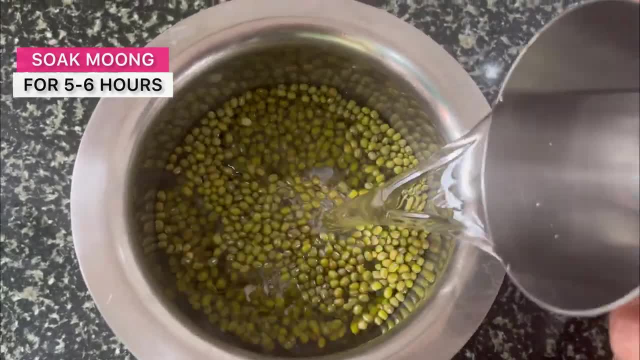 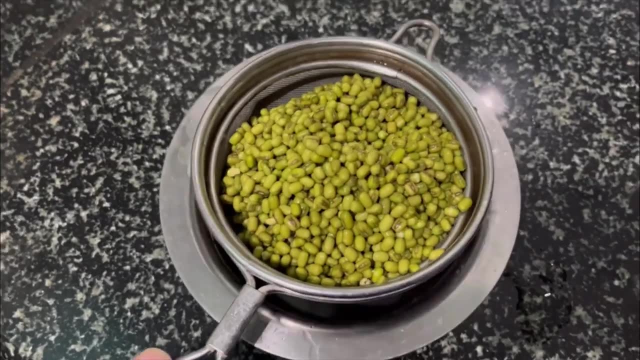 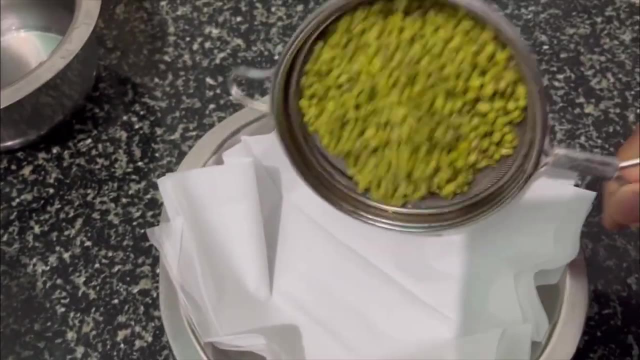 first to make the sprouts. we will soak moong dal for five to six hours. moong will swell up and started sprouting. now strain the water, take some tissue paper or any muslin cloth, put the moong dal on it and cover it well. keep it in dark place for 10 to 12 hours. after 10 to 12: 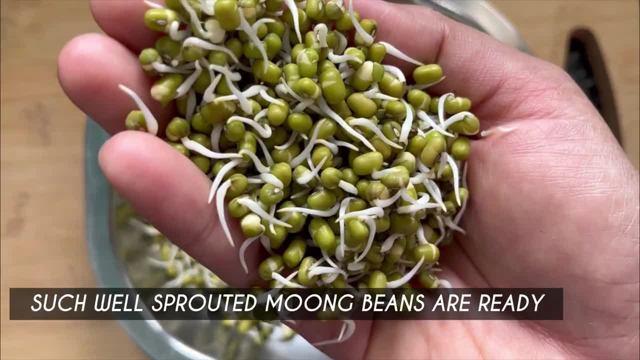 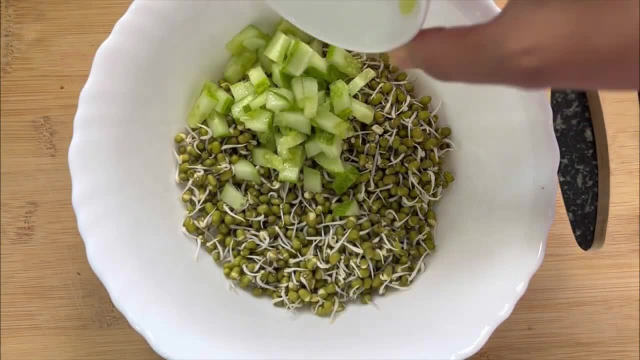 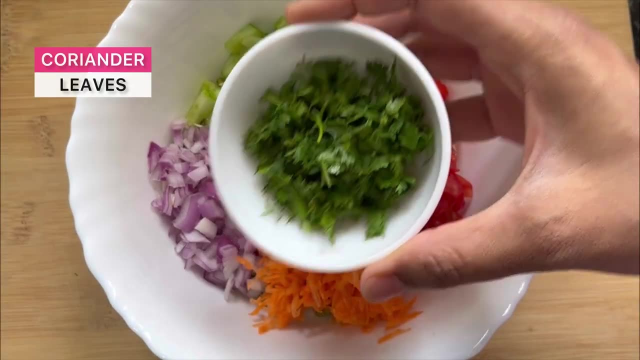 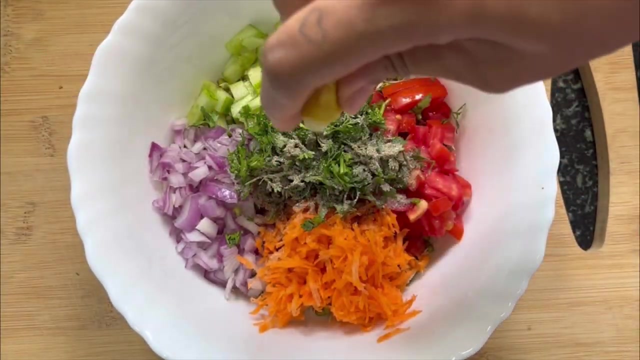 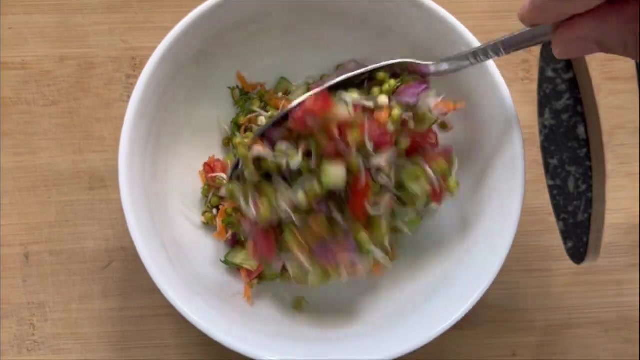 hours. such well sprouted moong beans are ready to make its tasty chaat. in a bowl, add one cup moong dal sprouts. add chopped cucumber, onion chopped tomato, grated carrot, chopped green chili, coriander leaves, rock salt, pinch of pepper, pepper, 1 teaspoon lemon juice. give it a good mix and it's ready, rich in protein.